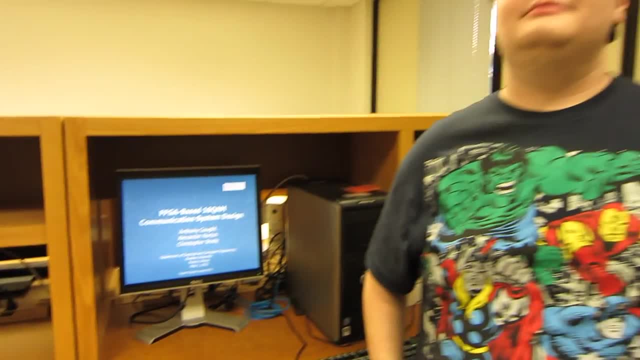 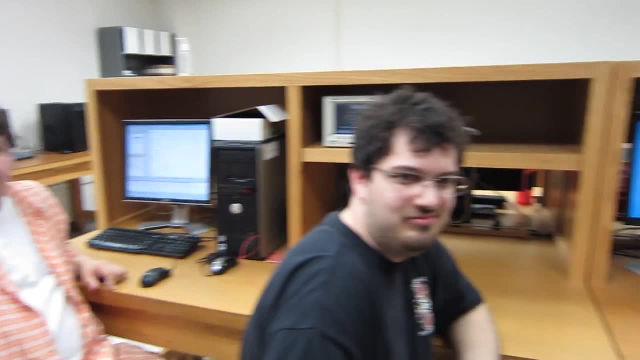 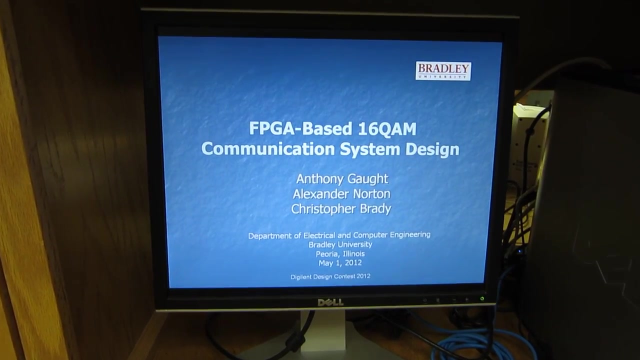 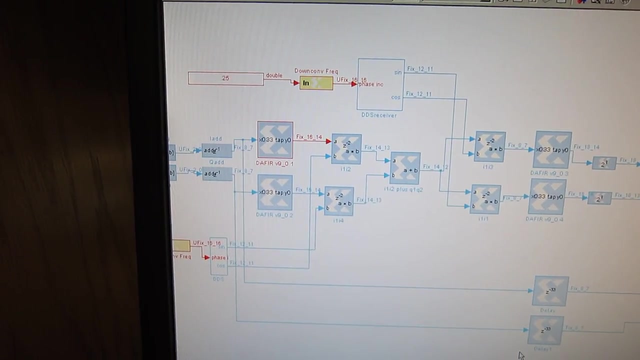 My name is Christopher Brady, My name is Lawrence Norton, My name is Anthony Gott. This is a report for our FPGA-based 16 QAM communication system design. We designed both the transmitter and the receiver. This is our Simulink model. As you can see, on the left we have a random symbol generator which we use MATLAB to generate random 4-bit symbols. 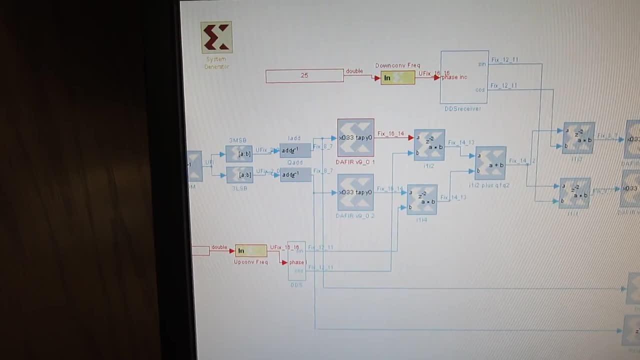 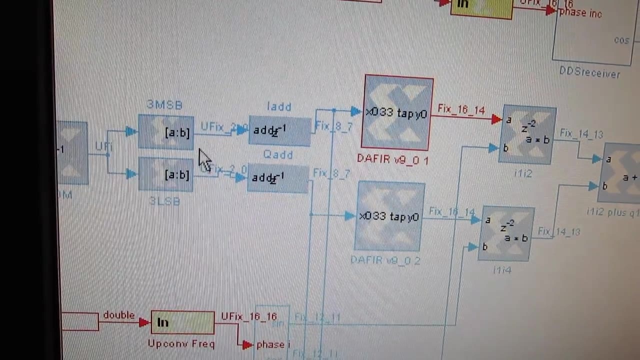 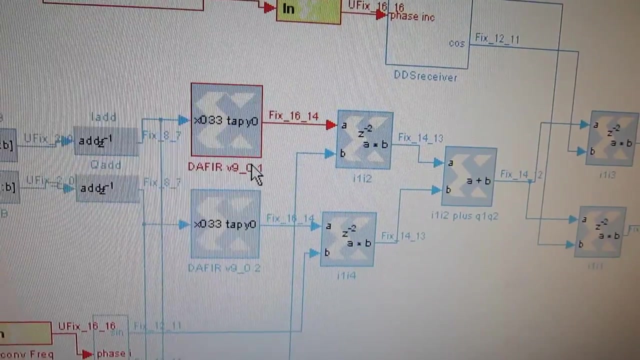 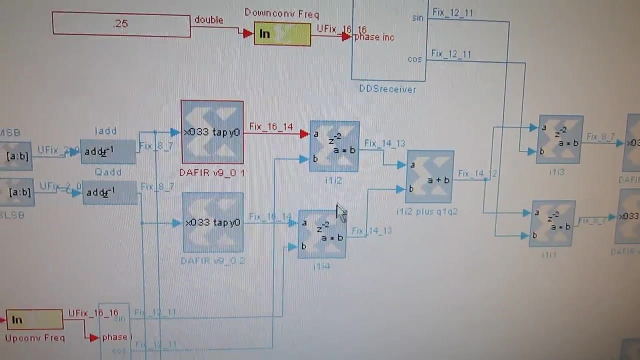 We then split them into the in-phase and quadrature components, which we then map to four levels. We then pass that through a square root raised cosine filter for pulse shaping. This is to both reduce the bandwidth and minimize the inter-symbol interference. We also upsample Here: we modulate the symbols by multiplying by sinusoidal carriers. 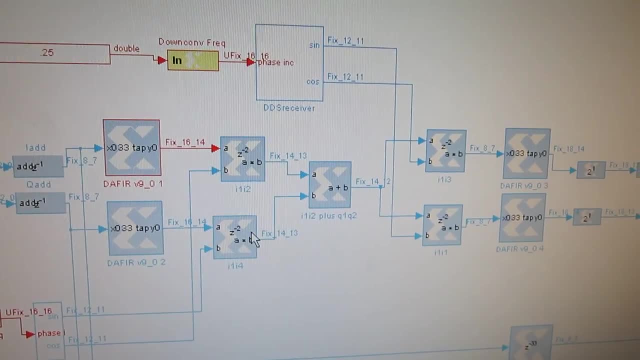 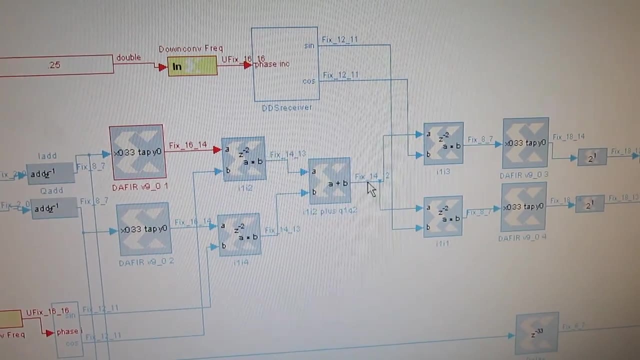 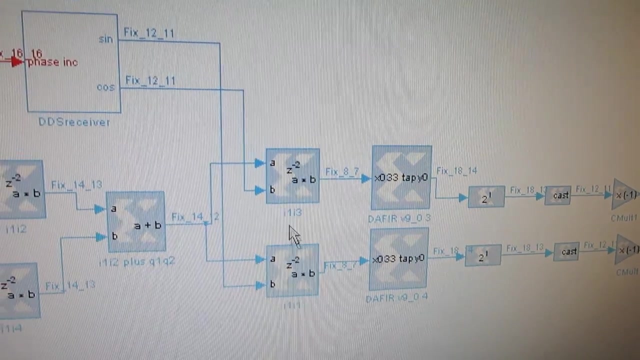 We multiply the in-phase by a cosine carrier and the quadrature by a sine carrier. We then combine those two for transmission. On the receiver side, we split the received signal into the two channels. We then demodulate it by multiplying again by the sinusoidal carriers. 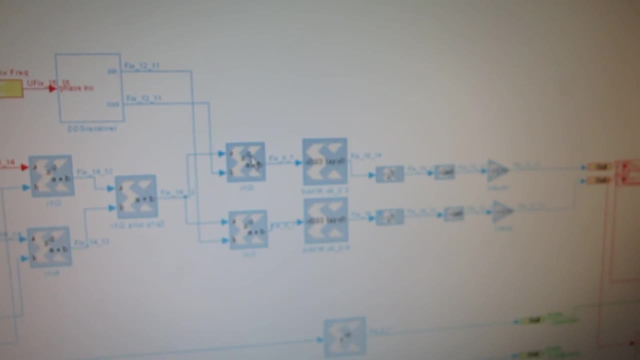 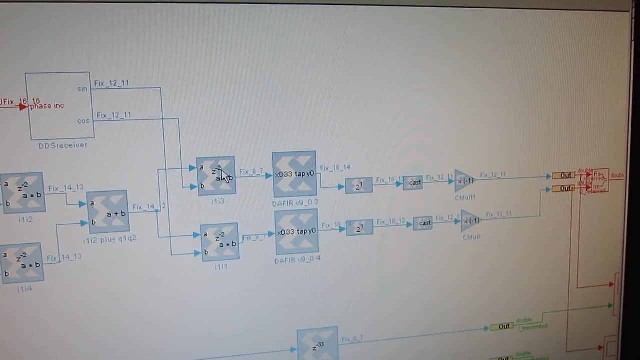 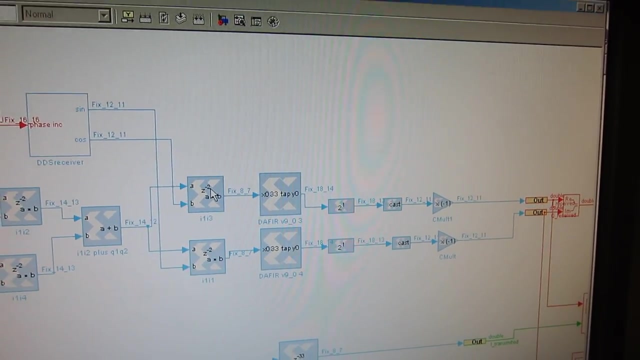 If the local carrier frequency is the same, the signal can be easily recovered. In an actual implementation, the carrier frequencies may be slightly different. If this is the case, a carrier correction hardware is needed, such as the phase lock loop. We have not implemented this for our project due to time limits. 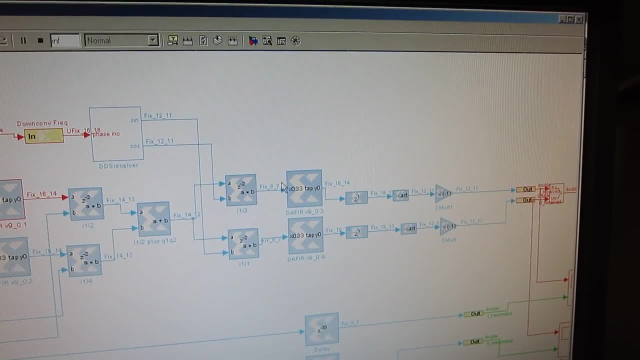 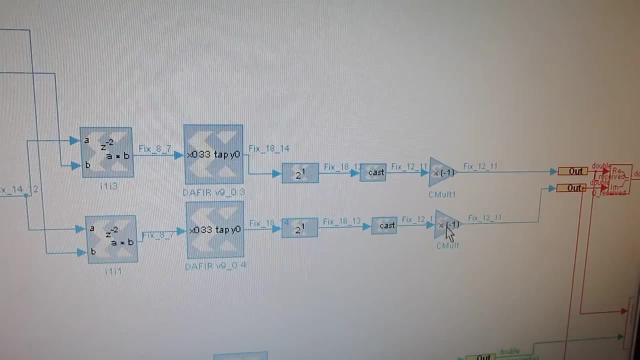 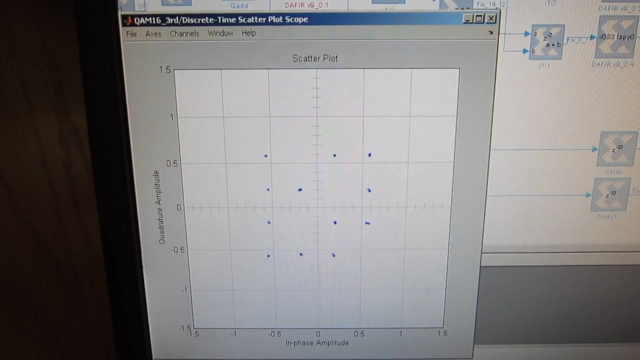 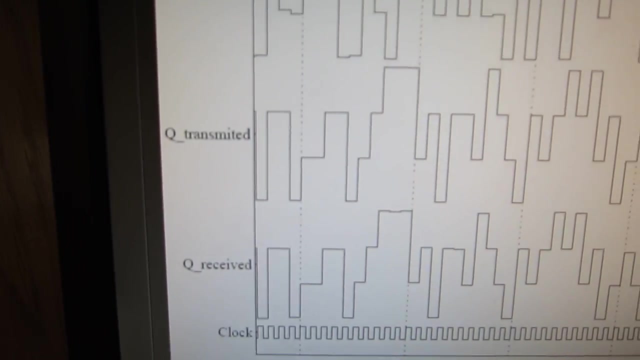 We then pass it through a matched square root raised cosine filter and downsample. We then output the recovered signal to the scatterplot. As you can see here, this is our scatterplot result. This is our in-phase and quadrature. received and transmitted symbols. 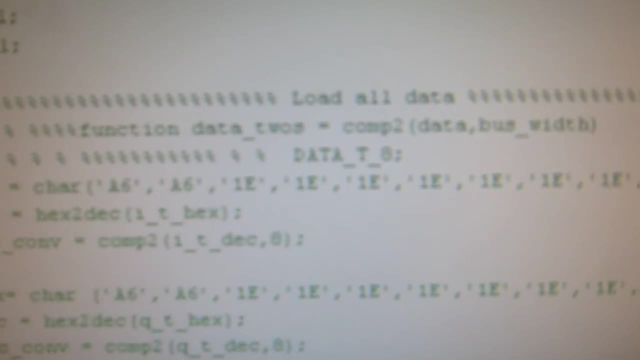 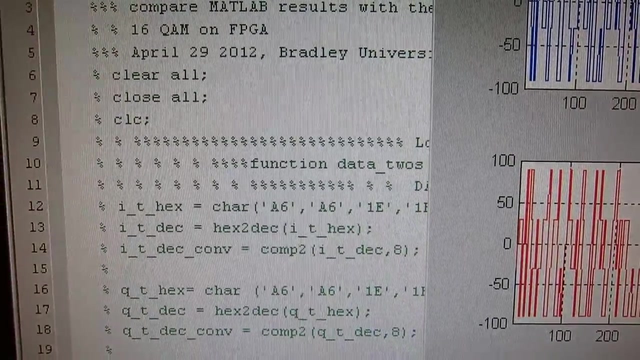 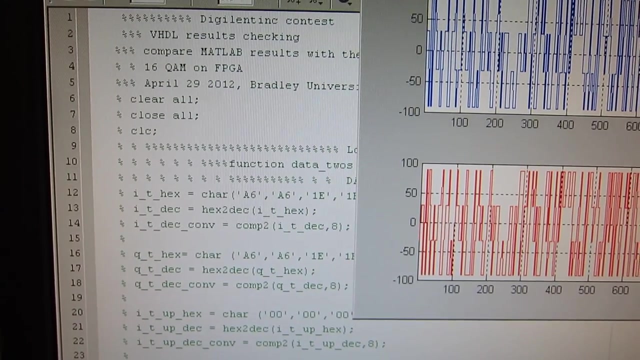 Next we will show you the hardware implementation results. We take our results from our implementation and save them to a text file. We then import that text file into MATLAB to compare with the simulated results. We then import that text file into MATLAB to compare with the simulated results. 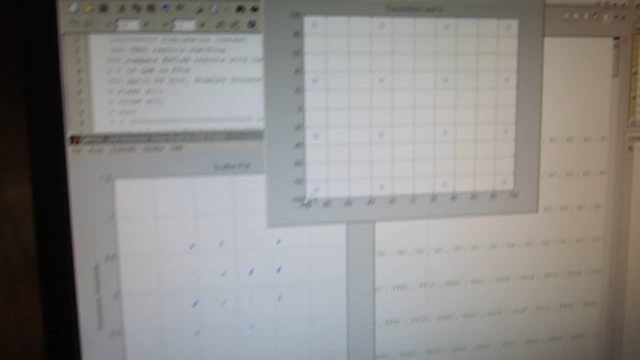 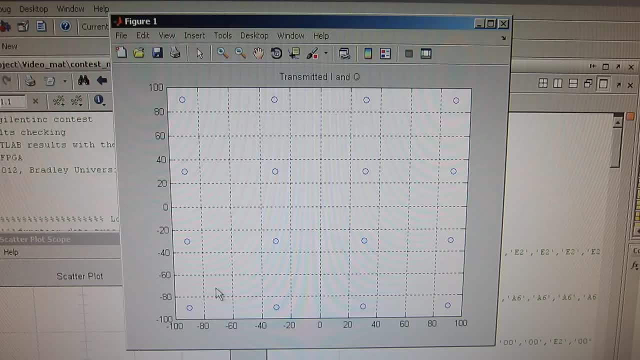 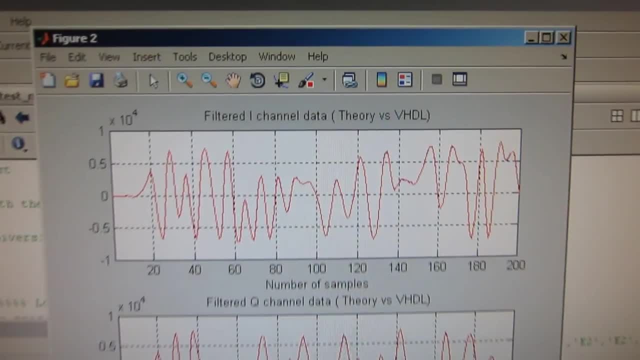 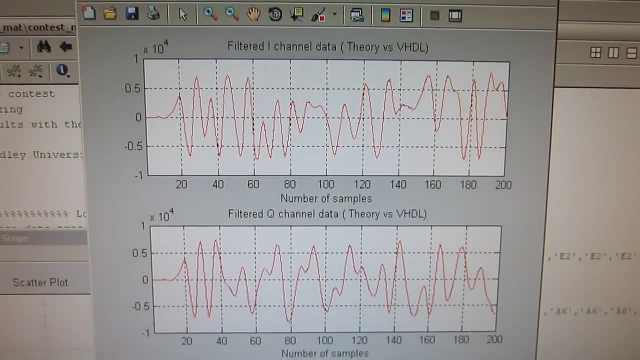 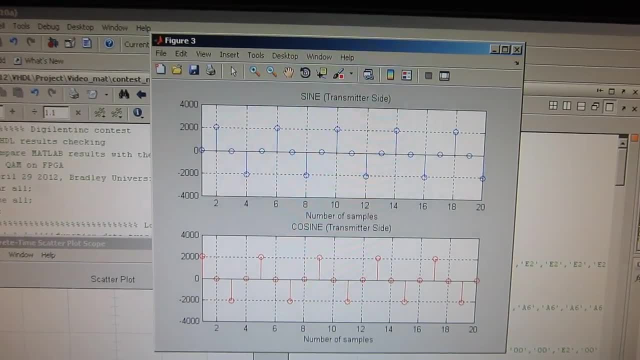 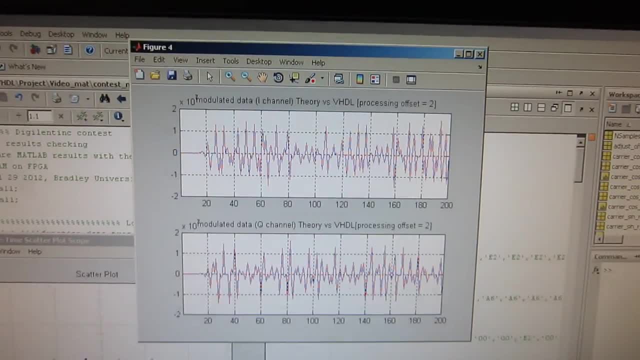 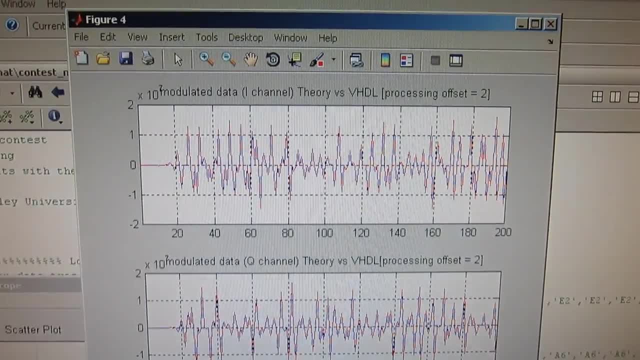 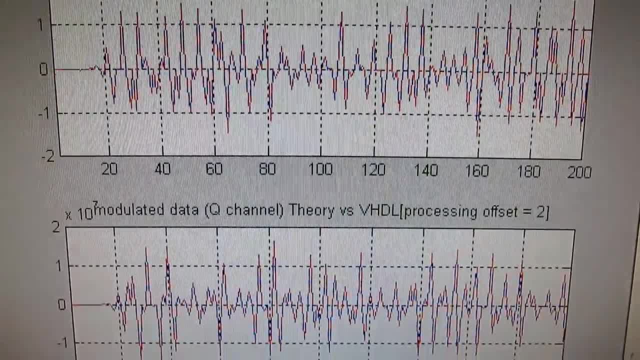 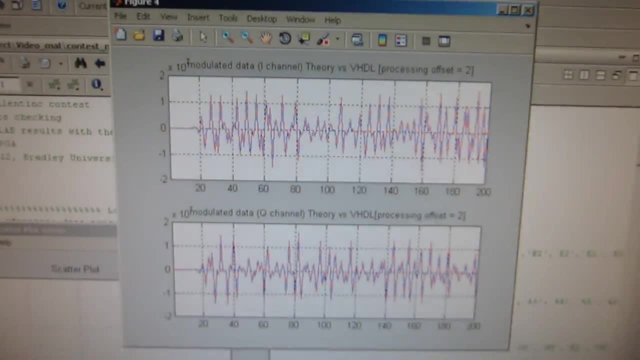 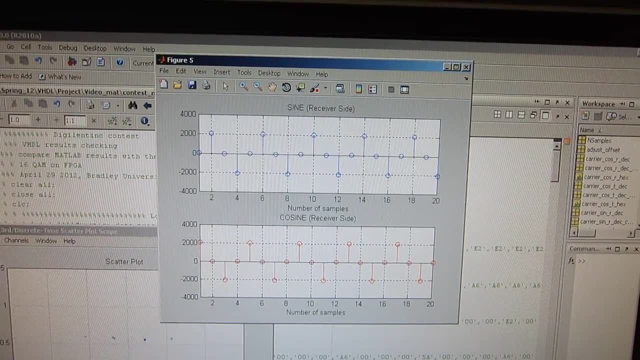 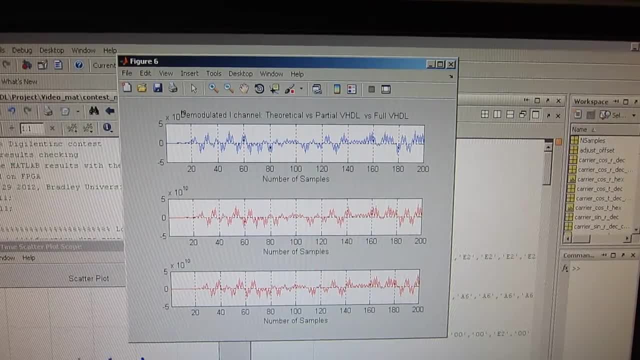 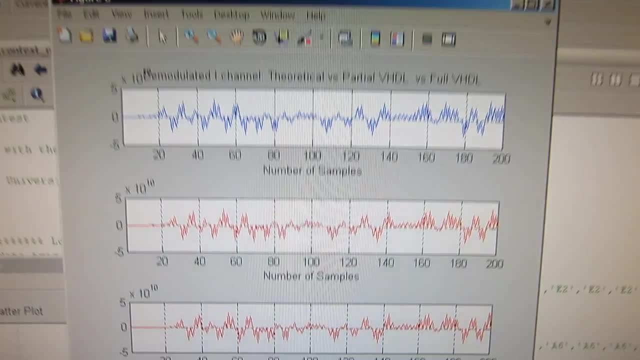 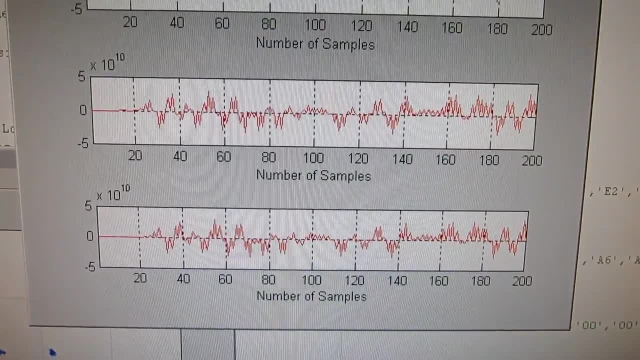 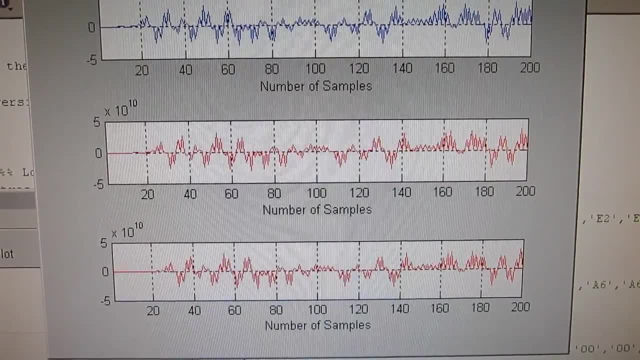 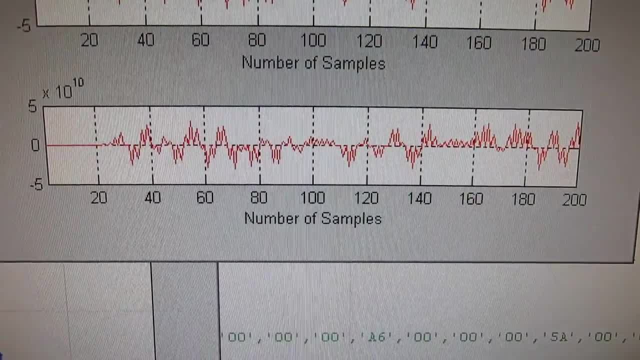 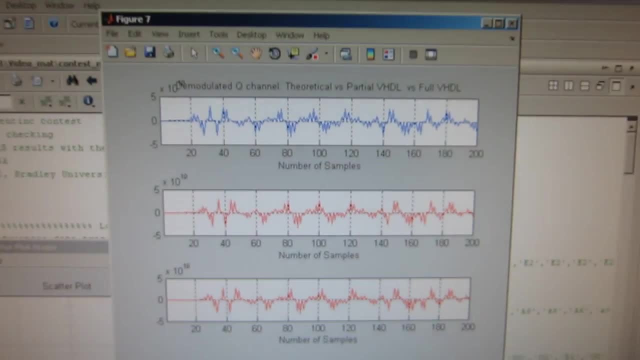 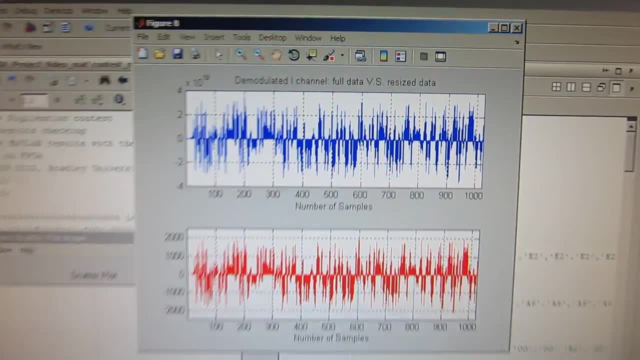 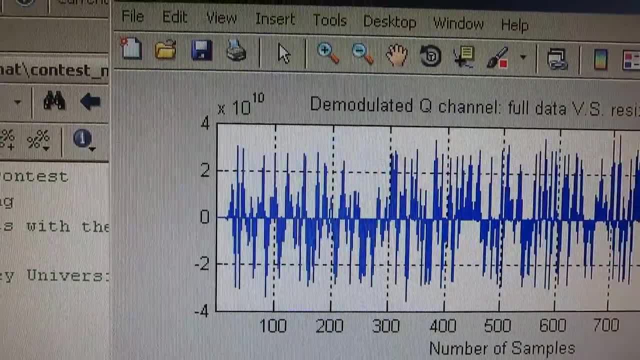 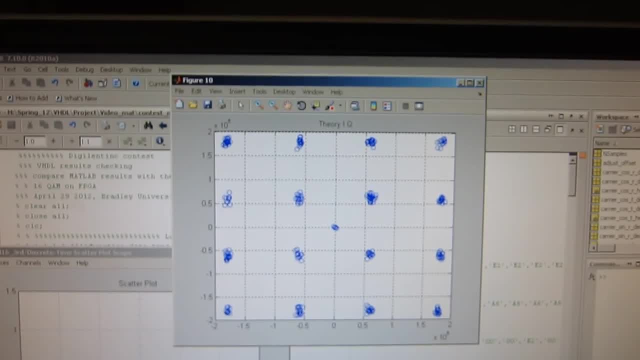 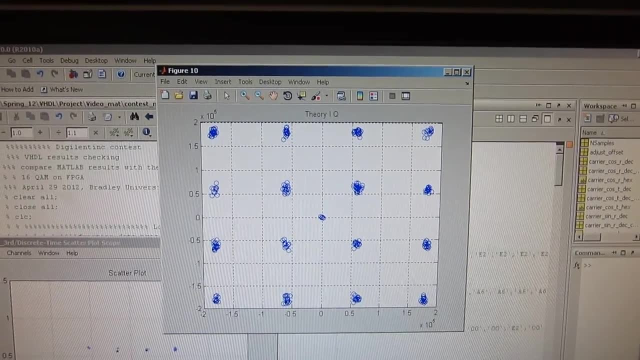 bottom for both the end phase and the quadrature. This is the MATLAB MASH filter demodulated VHDL signal. Note that a few initial zeros are shown on the scatterplot. This is due to some delay. These are the actual results we obtained. 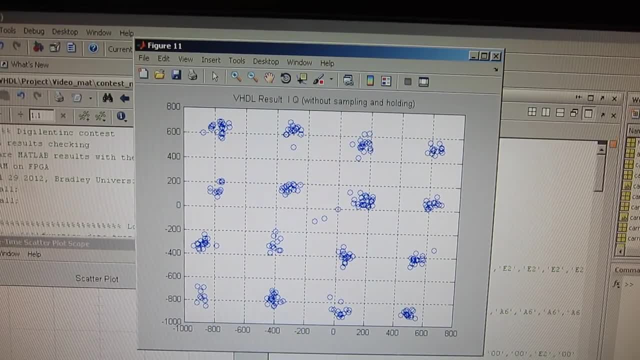 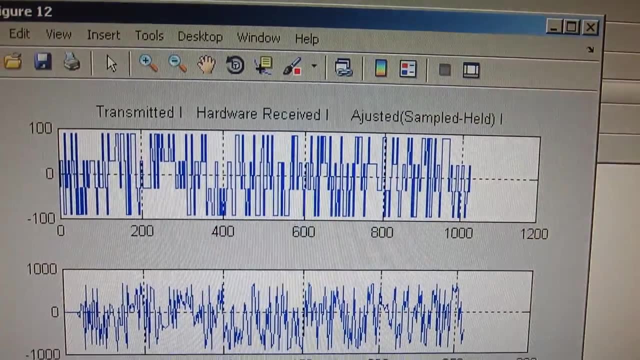 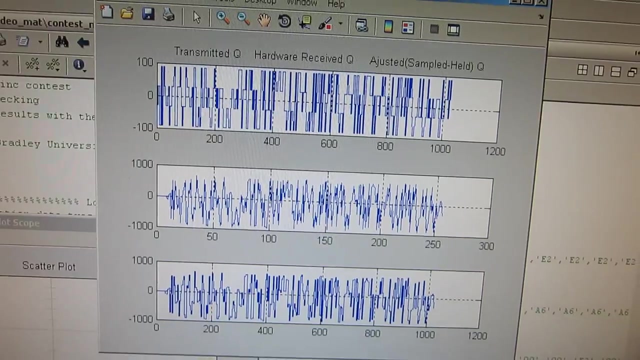 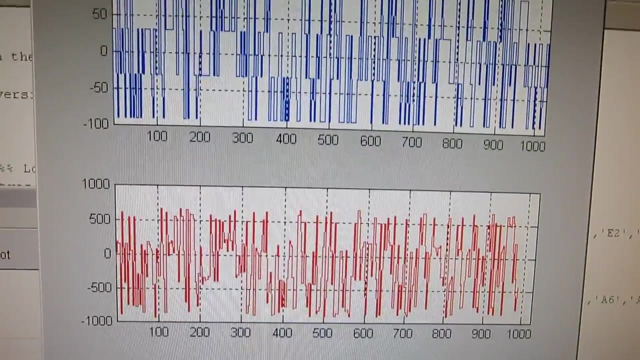 from the VHDL, As here you can see the infaise transmitted, received and then sampled signals. We obtained those for both the end phase and the quadrature components. Here we show the transmitted and received end phase and also quadrature. 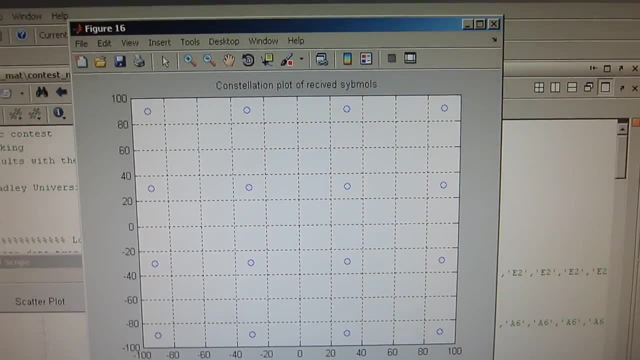 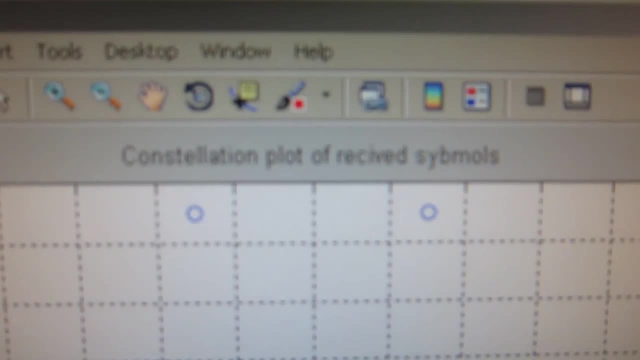 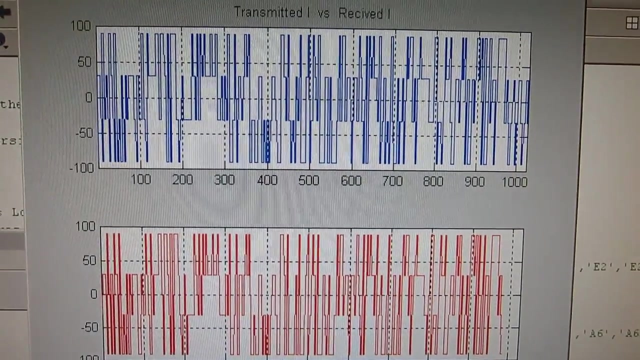 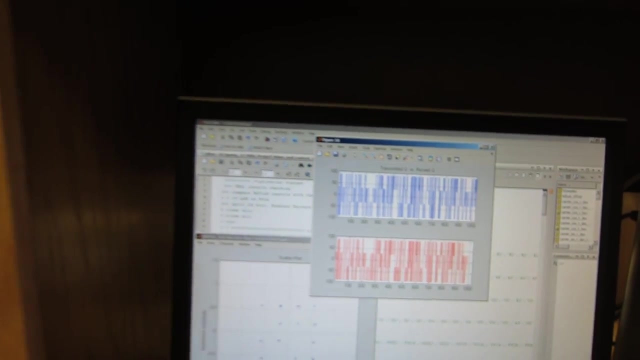 Here we use a thinker. It's a threshold device in order to increase accuracy for our recovery of the symbols. And when we use that, this is our received and transmitted end phase and then our received and transmitted quadrature. Next we move over to the actual hardware implementation. 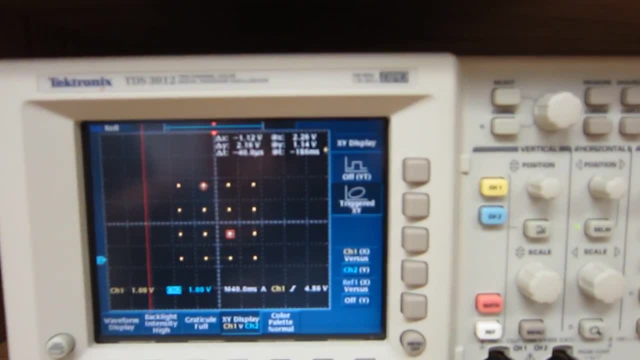 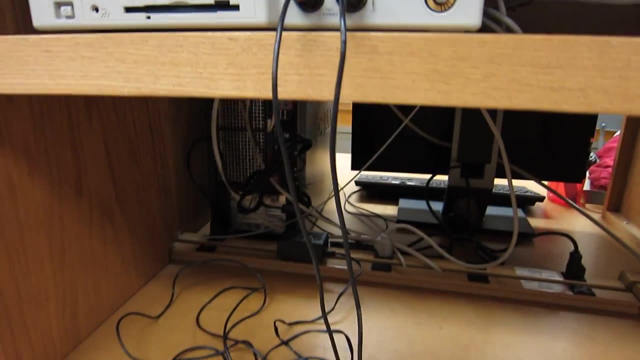 This is the results from our D-Day converter, and we also have the symbol generator here, And this is all being run directly on the Xilinx board. 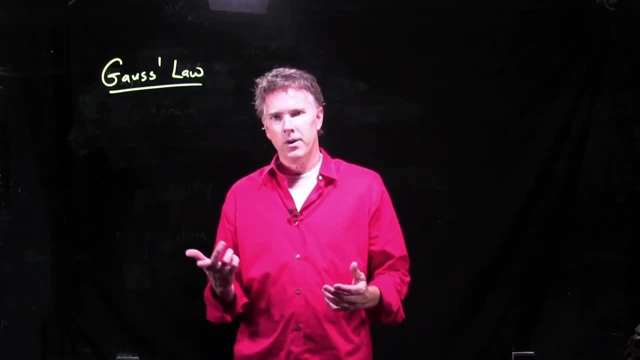 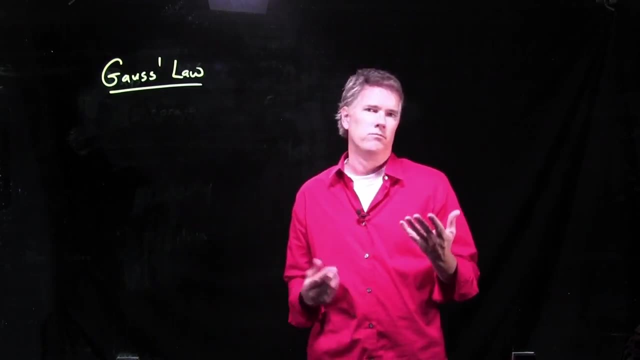 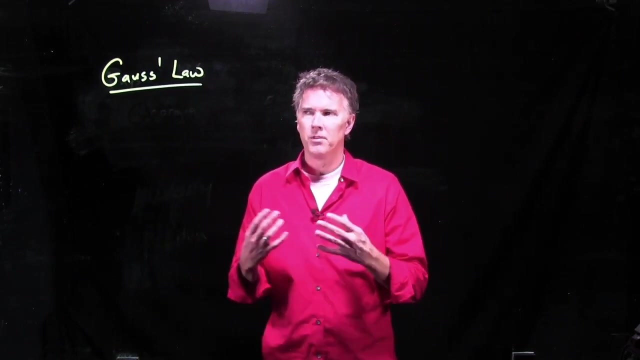 Hello class Professor Anderson, here Today we're going to talk about Gauss's Law. Gauss's Law is a great way to determine electric fields of rather complicated pictures, and Gauss's Law relies on some of the symmetry in the problem to help us understand.